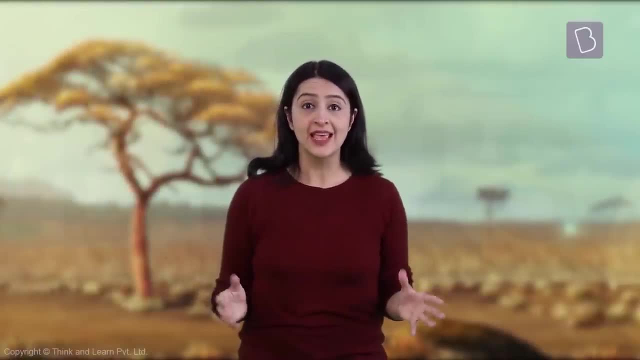 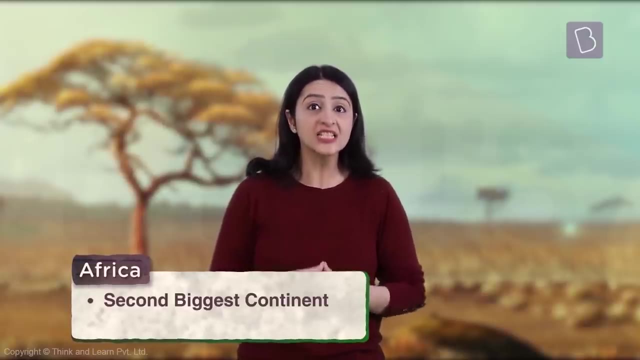 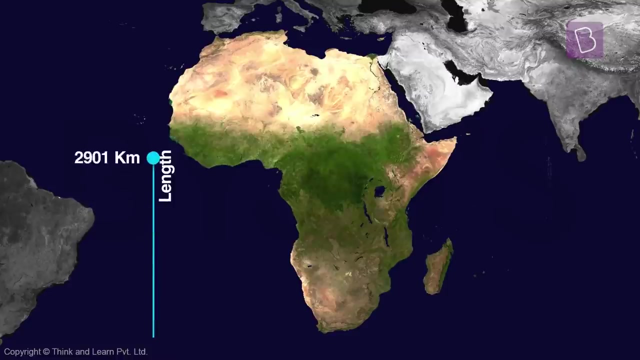 Africa is huge. It is the second biggest continent after Asia, covering a total area of 30.4 million square kilometers. The length of the continent is about 8000 kilometers. The width of the continent is about 7000 kilometers. The length of the continent is about 7400 kilometers. 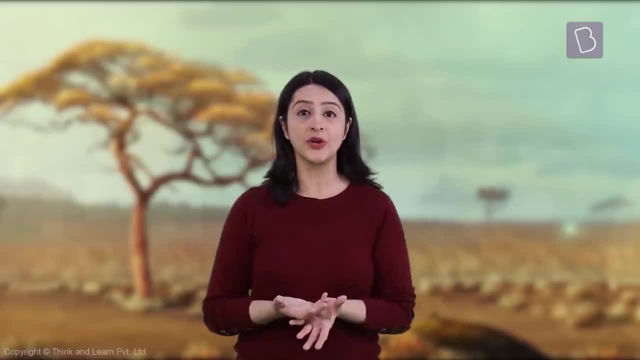 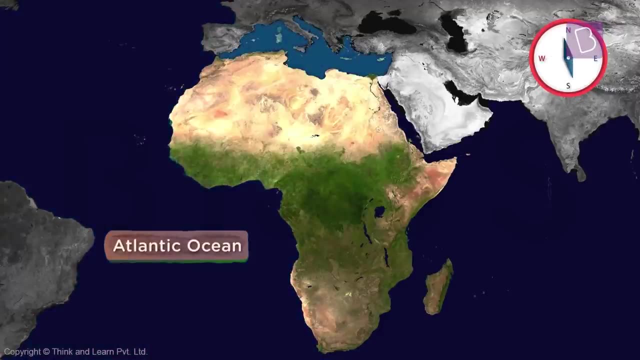 Africa is surrounded by large bodies of water on all sides. In the west it is bound by the Atlantic Ocean. In the north you can see the Mediterranean Sea. The northeastern side of the continent is bordered by the Red Sea. The eastern part of the continent is surrounded by the Indian Ocean. 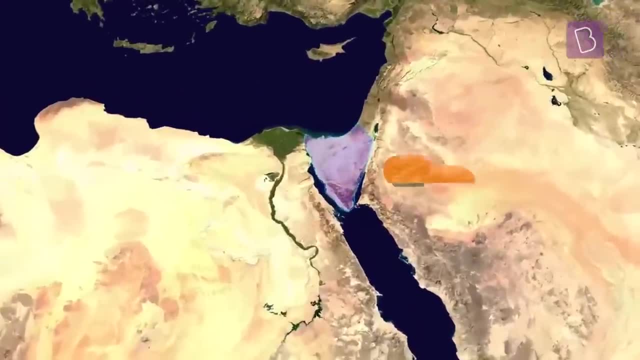 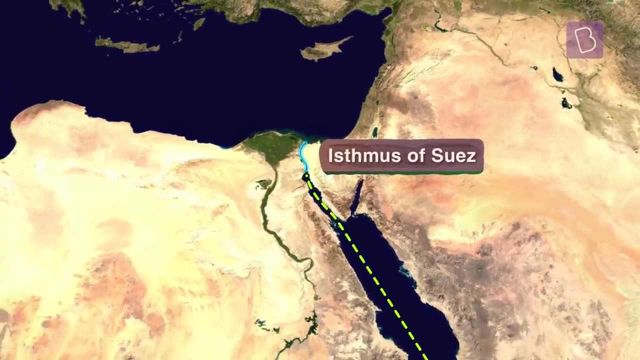 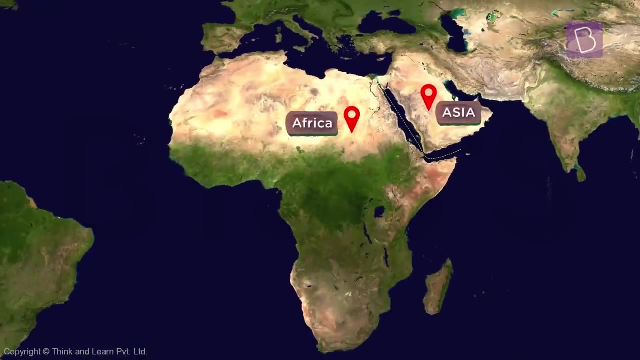 Africa is connected to Asia's Sinai Peninsula by a narrow strip of land called the Isthmus of Suez. The Isthmus of Suez joins the two land masses of Asia and Africa. The famous Suez Canal is cut through the Isthmus of Suez. 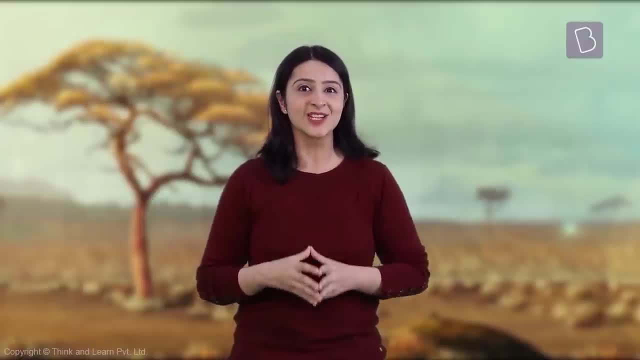 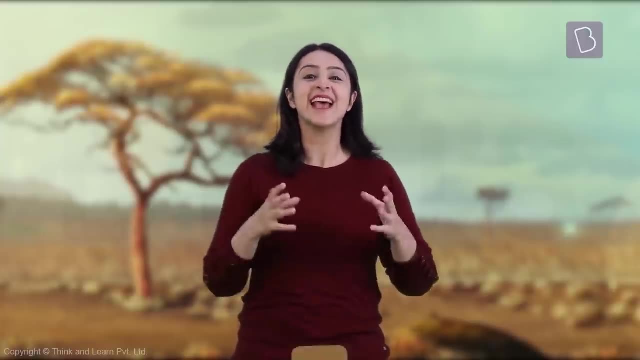 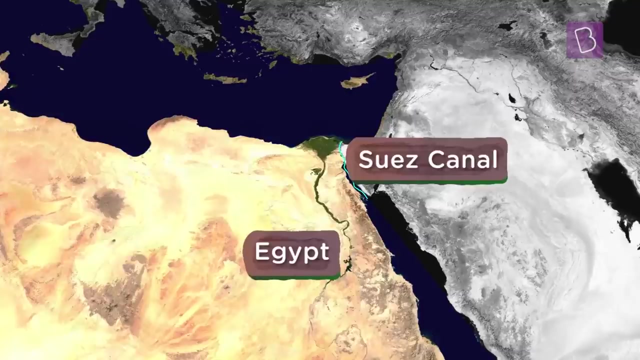 By now, many of you would have guessed the location of this Isthmus. Yes, No, Alright, I'll tell you: It's in Egypt. The Suez Canal is the biggest man-made canal linking the Mediterranean Sea and the Red Sea. 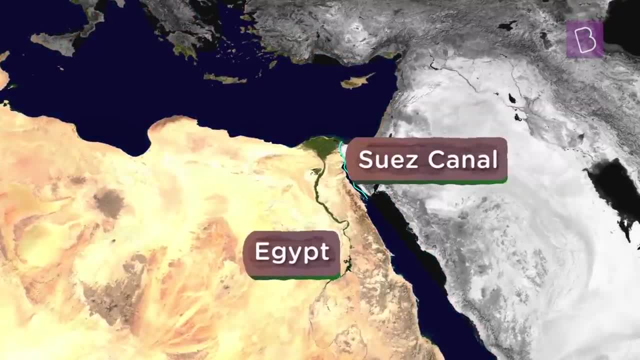 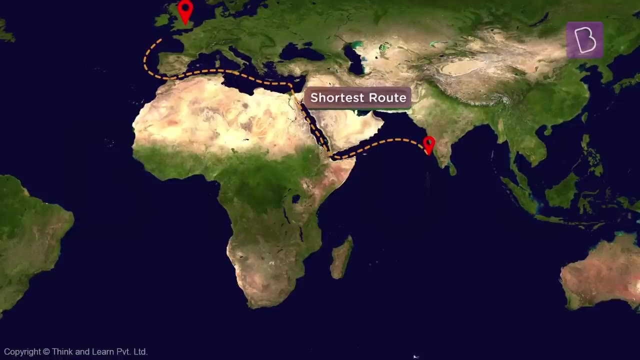 The Suez Canal is one of the busiest sea routes in the world, So all the efforts put into building this canal was totally worth it. It connects Europe with Asia. It connects Europe with Asia, But by a short distance. Sailors or traders of Europe who want to sail to Asia need not travel around Africa to reach Asia because of the Suez Canal. 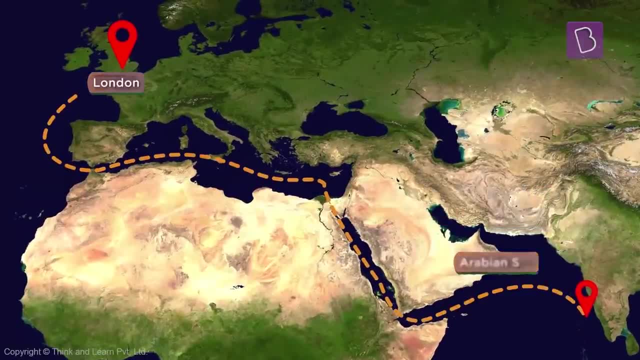 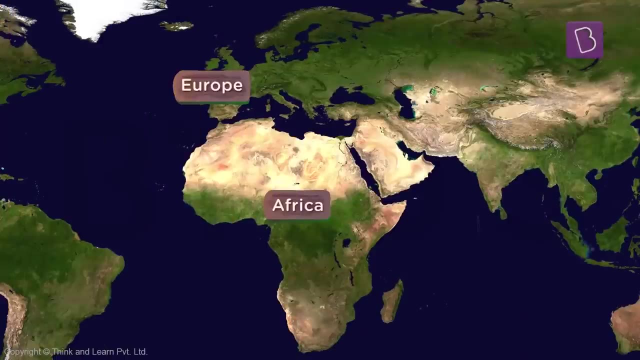 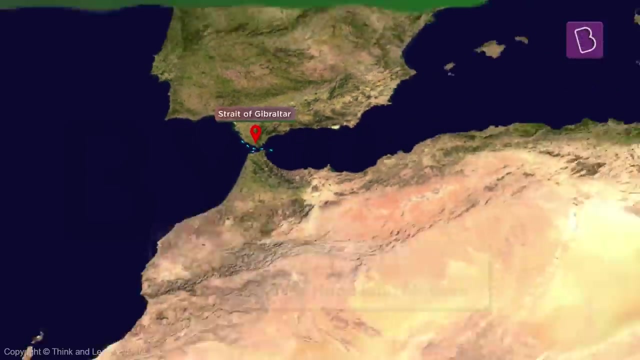 A ship traveling from London to the Arabian Sea would save approximately 8,900 kilometers of journey because of the Suez Canal. That's right, Awesome, isn't it? Asia is separated from Europe by the Strait of Gibraltar. A strait is basically a narrow water body that separates two huge land masses. 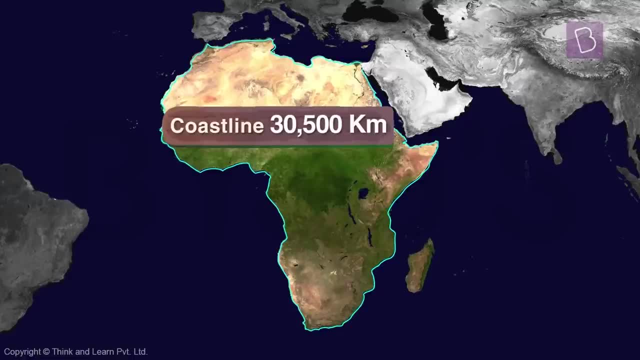 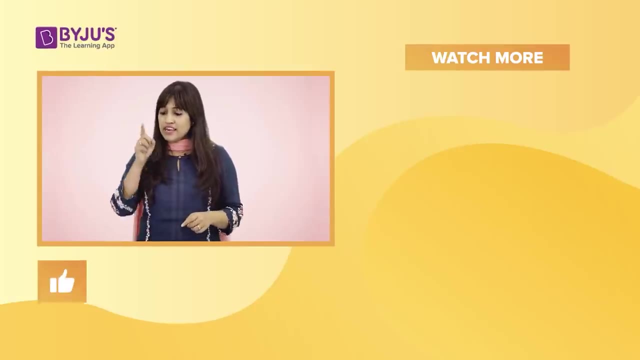 The coastline of Africa stretches for 30,500 kilometers. In spite of such a long coastline, the continent poses challenges to outsiders. If you like this video and want to watch many, many more amazing videos like these. If you like this video and want to watch many, many more amazing videos like these. like and subscribe to our channel now. 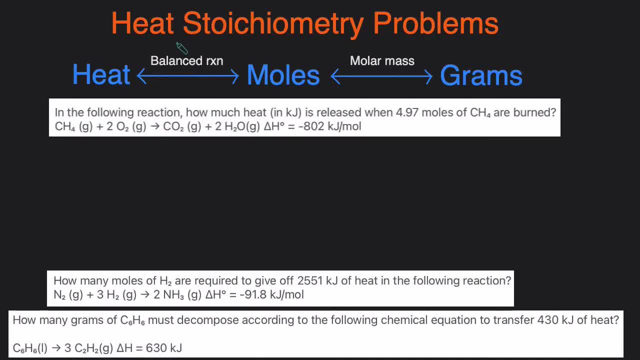 Hey guys, it's Mike from Conquer Chemistry. In today's video we'll be going over how to do heat stoichiometry problems. Heat stoichiometry problems will usually involve a chemical reaction with the enthalpy or the delta H that's given. 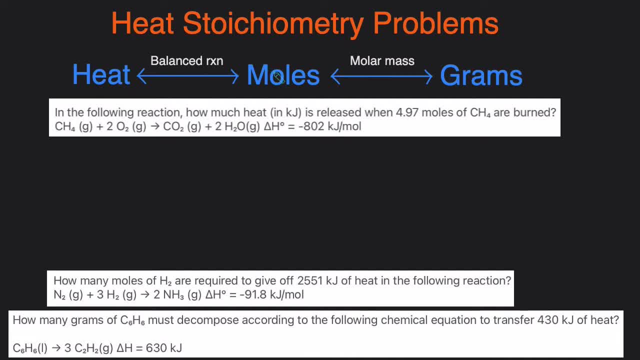 and you'll either be asked to solve for the amount of heat, the moles or the grams. And I have the flow chart written right here and we have three example problems, so let's jump into it and work through these. And the first question asks, in the following reaction: how much heat in kilojoules is released when 4.97 moles? 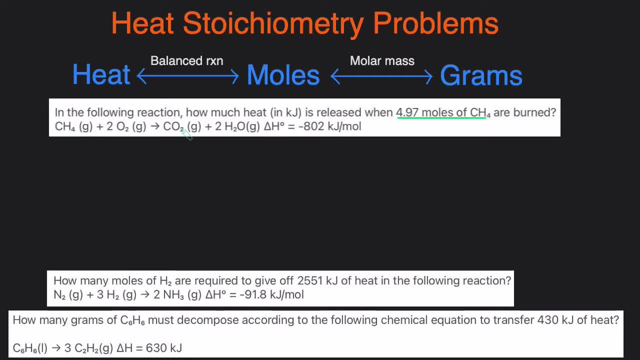 so you're given the moles are burned, and then you're also given this chemical reaction. So in this chemical reaction you can see when we burn 1 mole of CH4, it's going to release 802 kilojoules of heat. 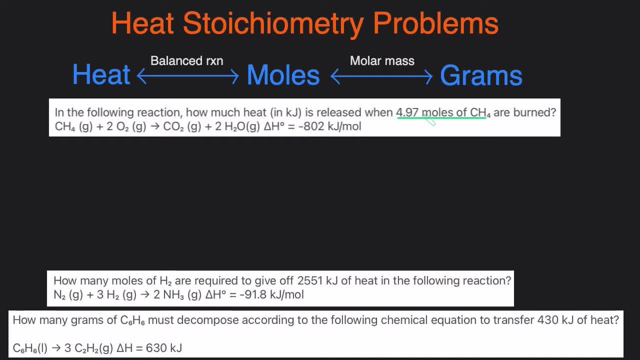 The negative just means the energy is going to be released. So we're burning 4.94 moles and it's asking for how much heat will be given off. So we always start with the number that's given. That's not in the chemical reaction. 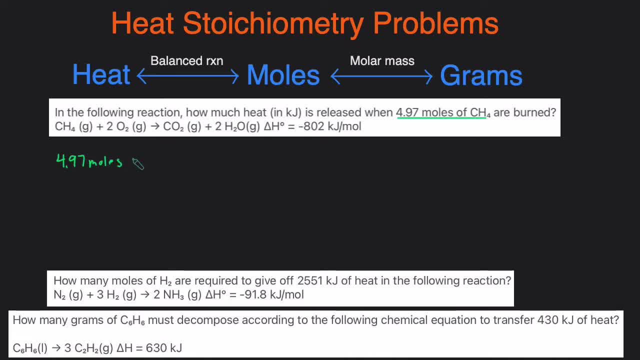 4.97 moles of CH4, and then we're going to multiply it by the conversion factor and you can see that we have moles and we want to get to heat, which is in kilojoules. So we just need to look at the chemical reaction. 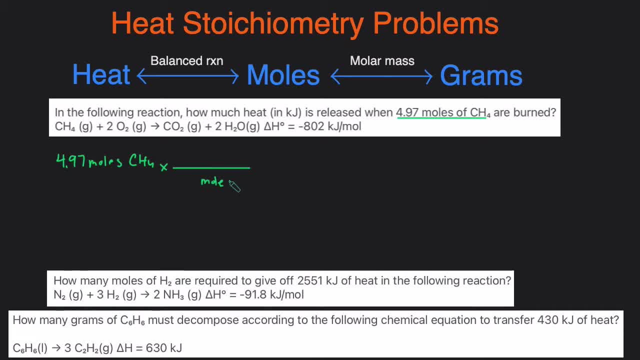 Whatever goes on top has to go on the bottom so it can cancel out. So we'll put moles of CH4 on the bottom and whatever we're trying to get to will go on top. We're trying to get to kilojoules, so we'll put kilojoules on top.